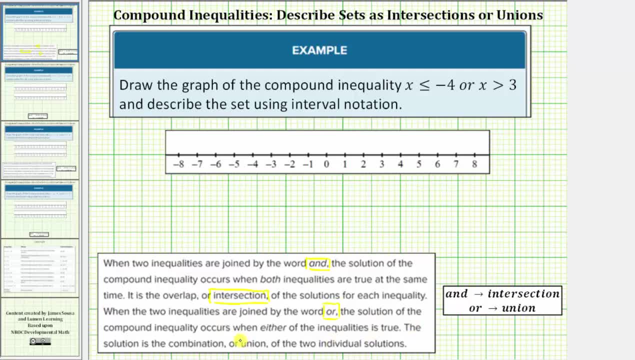 inequalities is true. The solution is the combination or union of the two individual solutions. So the main thing to remember is for the word, and we're looking for the intersection For the word, or we're looking for the union of the two intervals. So for the first step, we want to graph each 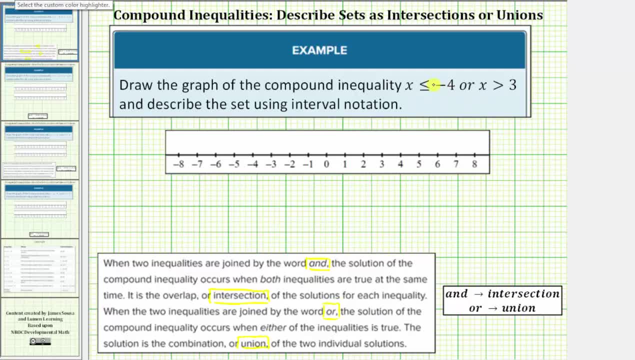 interval on the number line. Let's first graph x: less than or equal to negative four. Notice, negative four is in this interval. So we make a closed circle or closed point on negative four and because it's less than or equal to negative four, we have an arrow to the left approaching negative infinity. 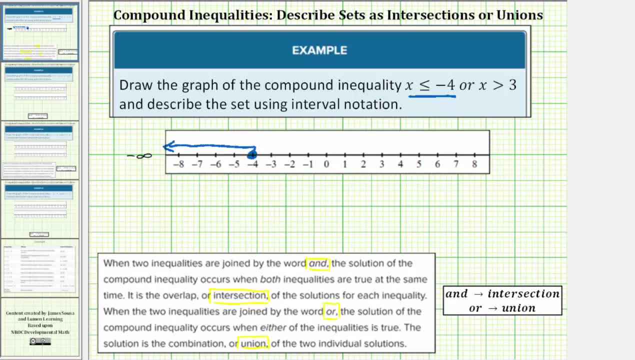 This will be helpful when we give the interval notation. Now we want to graph x greater than three. Notice, three is not in the interval and therefore we make an open circle or open point on three. And because it's greater than three we have an arrow to the right, approaching positive infinity. And now, because we 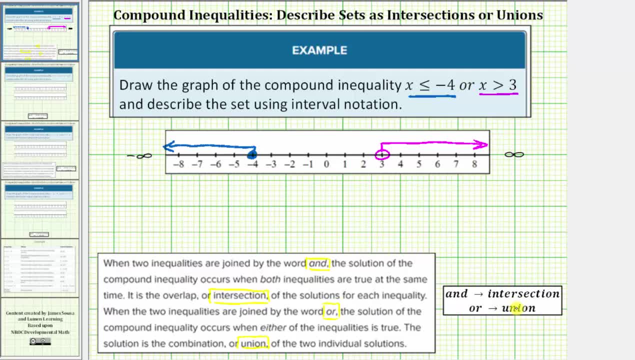 have the word or we're looking for the union or the combination of these two intervals, which means these two intervals are the solution to the compound inequality. And now we want to describe this set using interval notation. Because we have an interval on the left and on the right, we'll have two interval notations. 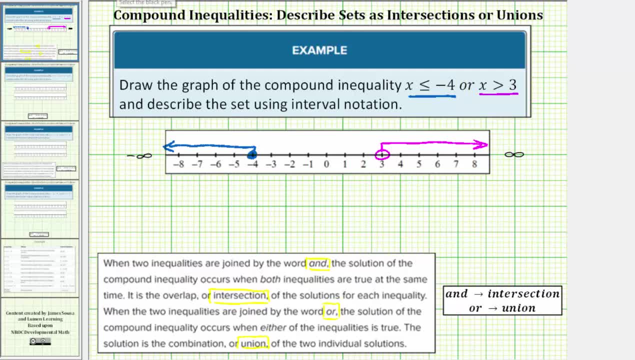 connected with the word or or u for union. So the interval on the left would be all real numbers less than or equal to negative four. So for interval notation we'd have negative infinity comma, negative four. The interval includes negative four. We have a bracket to the right. 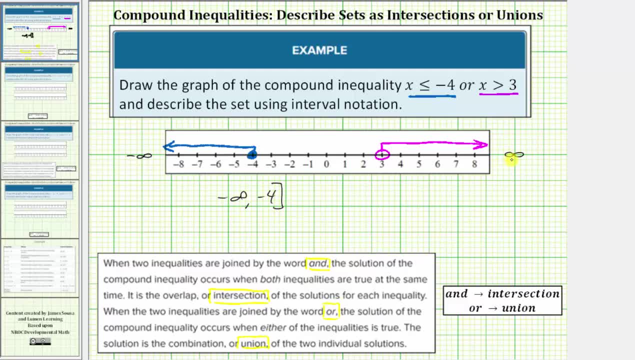 of negative four, And for negative infinity and positive infinity We will use a random parenthesis. We have an open parenthesis to the left of negative infinity, And then we'll use u for union. Sometimes you'll see the word or- And then we have the interval from three to infinity. 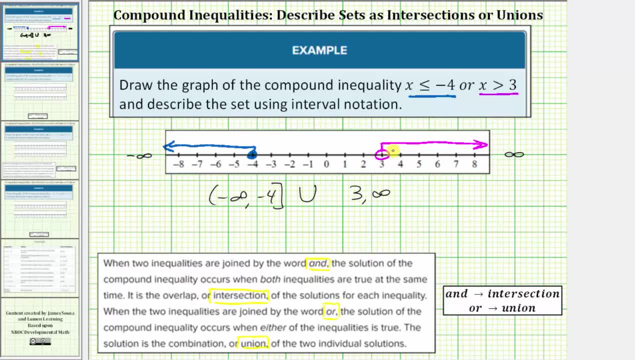 So three comma infinity. Three is not in the interval, So we use an open parenthesis to the left of three and a closed parenthesis to the right of infinity. This is the graph of this solution And here's the solution expressed using interval notation. 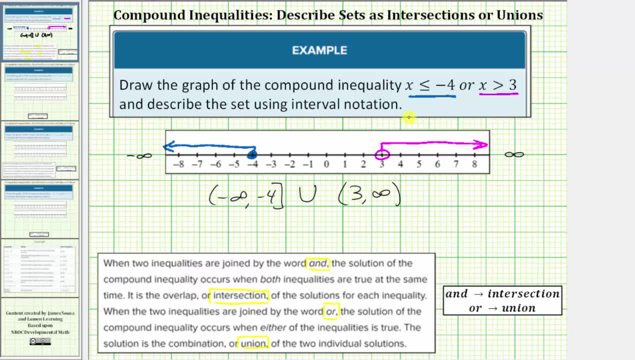 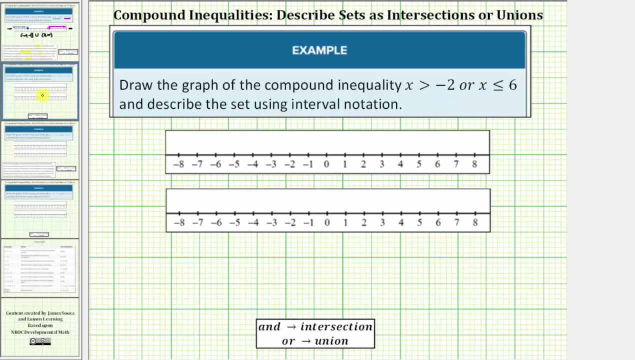 One thing to be careful about, though, is that not all compound inequalities with, or will have a solution that looks like this, So let's look at a second example. The directions are the same, So let's first graph both inequalities on the same number line. 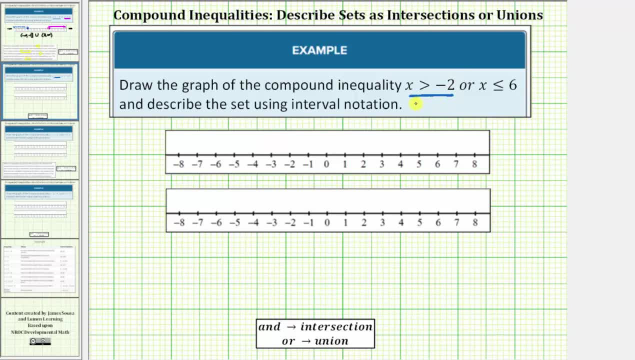 So we'll first graph x greater than negative two. Negative two is not in the interval. We have an open circle on negative two Arrow to the right. So here's all real numbers Greater than negative two. Now we graph x less than or equal to six Six. 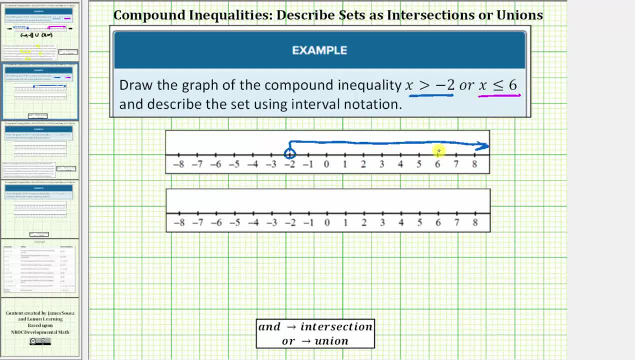 is in the interval. So we make a closed circle or closed point on six And it says x less than or equal to six. We have an arrow to the left And again to the right: we're approaching infinity. To the left, we're approaching. 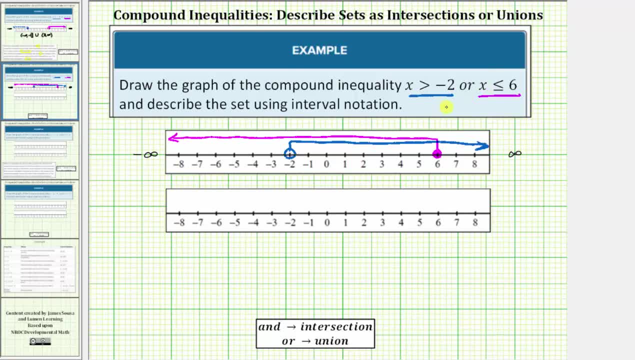 negative infinity. Now this is an or compound inequality. So the solution is a union where the combination of these two intervals, And notice how every number on the number line is graphed at least once, Which means the solution would be all real numbers. 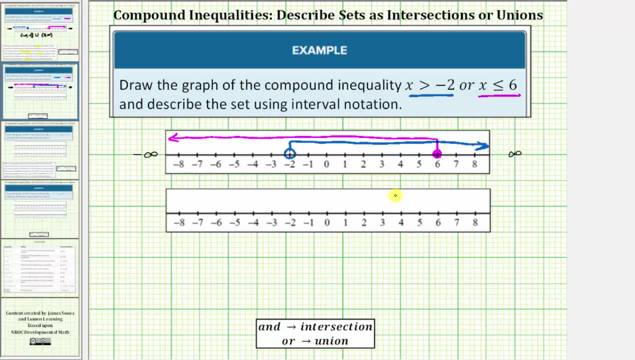 So, to graph all real numbers, we graph the entire number line approaching positive infinity to the right and negative infinity to the left. So this first number line shows our work. This is the graph of our final answer. Now we need to express this using interval. 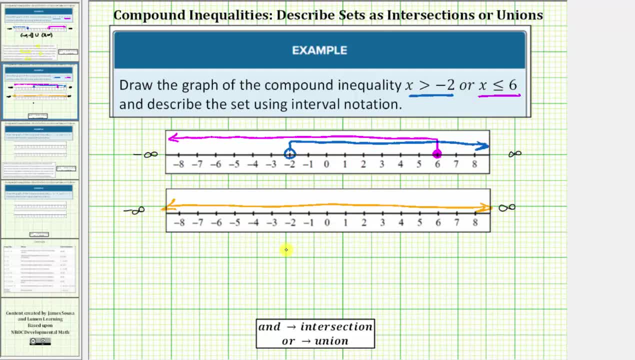 notation. So to the left we approach negative infinity comma. To the right we approach positive infinity, And for negative and positive infinity we always use a random parenthesis. So we have an open parenthesis to the left and a closed parenthesis to the right. 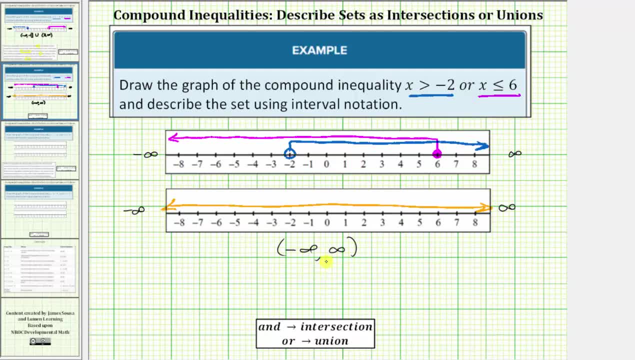 This is how we express all real numbers using interval notation, So it is important that we're able to interpret what union means when graphing a compound inequality with the word or. I hope you found this helpful, Thank you.